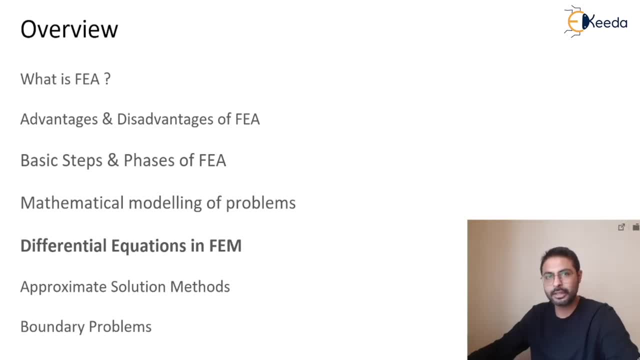 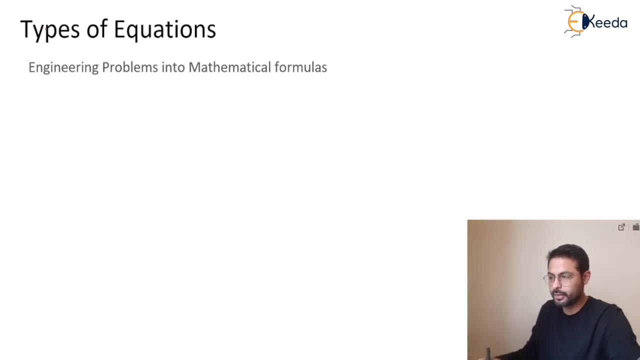 And how an engineering problem can be converted into a mathematical formula. So let's understand what is differential equations in FEA. So let's get started. So any engineering problem can be converted into mathematical formulas. You might have seen formulas like this. Yes, you guessed it right. 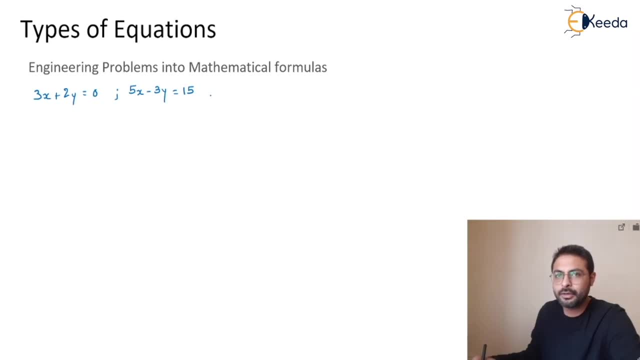 These formulas are known as algebraic formulas And these algebraic formulas are used to solve various problems like age related problem, or we want to predict some cost or any other general terms in day to day life. But what if some physical phenomena is changing over time? 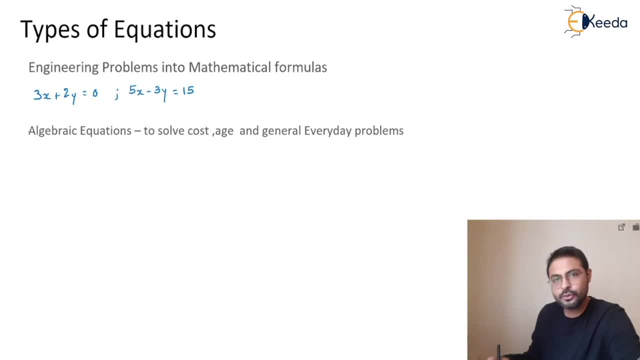 So that thing is known as derivative. For example velocity v. What is velocity? Velocity is nothing but the change in displacement in any one direction. Let's say x over time. It is also denoted by delta x, by delta t Or first derivative of displacement. 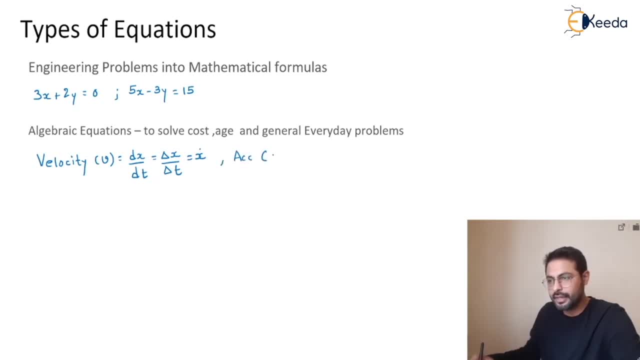 Same for acceleration. Acceleration is rate of change of velocity. That is derivative of velocity. So a is equal to dv by dt. It is also written as del v by del t, Or it is also represented by second derivative of displacement. So any physical quantity which is changing over time or any other phenomena is known as derivative. 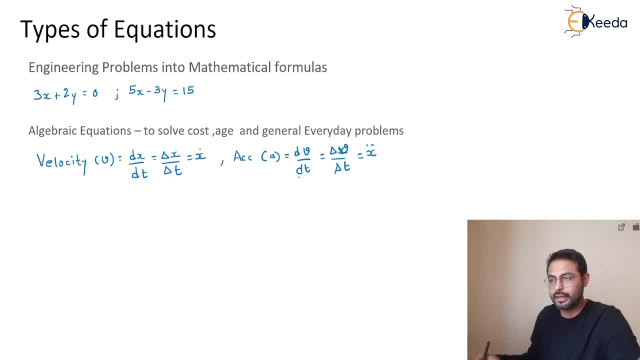 And any equation which carries this kind of derivatives are known as partial differential equation. So these partial differential equations are nothing but the equations of the differential equation, But the equation which is having some derivative inside it. And this differential equations are everywhere, Like in biology, if we want to find some spread of bacteria. 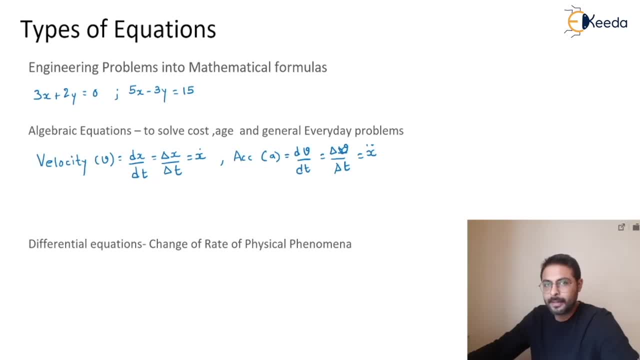 So the growth rate of bacteria can be represented by this kind of equation, Or, in any chemical reaction, How rapid the reaction is going to do, Or how the decay of carbon in any reaction That is represented by differential equation In physics. if you want to find out force. 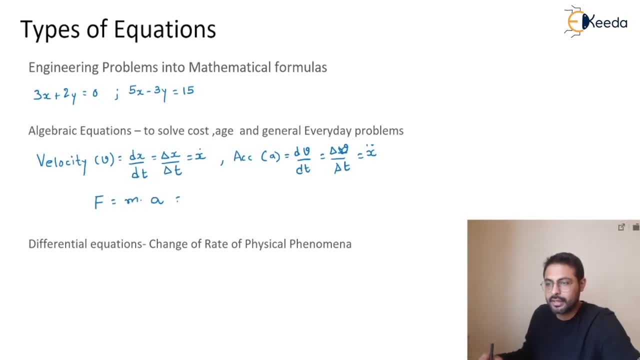 Force is equal to mass, into acceleration, Where acceleration is nothing but the second derivative of displacement. So d square, x by dt square. So in the equation of force itself It is the differential equation. So these differential equations are used to represent various physical phenomena in engineering field. 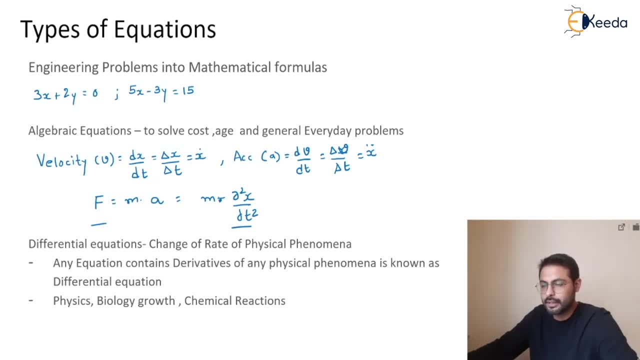 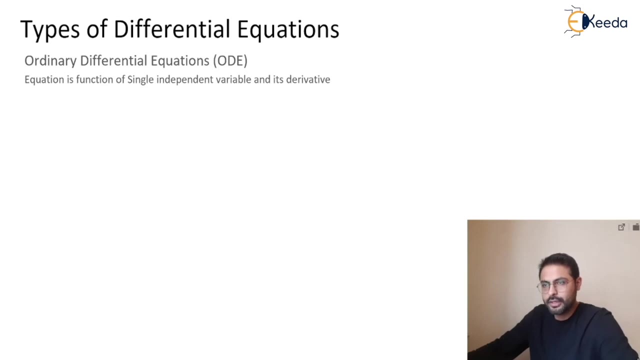 For example, physics, biology and chemical reactions. So let's understand differential equations in detail. Basically, there are two types of differential equations: First is ordinary differential equation And second is partial differential equation. So what is ordinary differential equation? To understand it better, 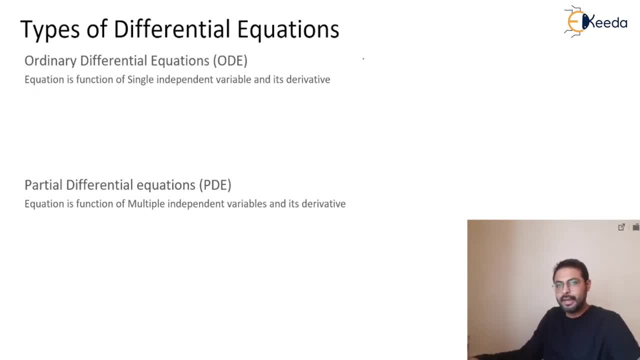 First we have to understand What is dependent variable and independent variable. You know the general notation, Which is x, y and z. This is the spatial coordinate representation. These are the spatial coordinates And time. Now you know. 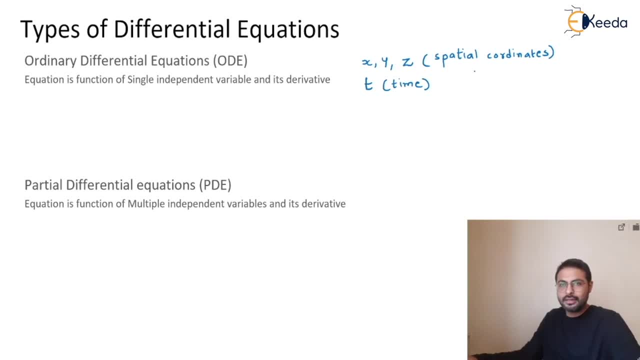 The spatial coordinates does not depend on any other variable, Or the time Time also does not depend on any other variable, So these two Are known as Independent variable, While, As we have seen, Velocity Depends on Spatial coordinates like x and time. 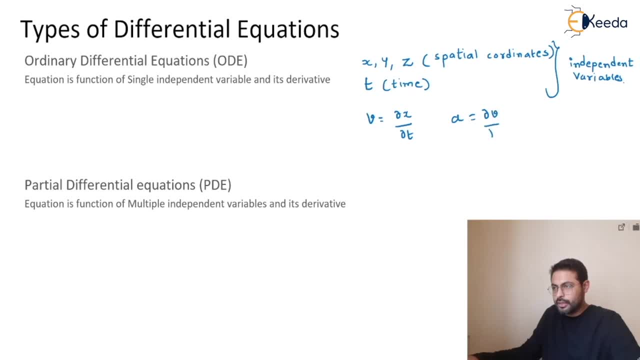 As well as acceleration. This also depends on velocity and time, So this kind of Variables are known as Dependent variable. So now you know Dependent variable and independent variable. If Any equation Is having Only single independent variable, 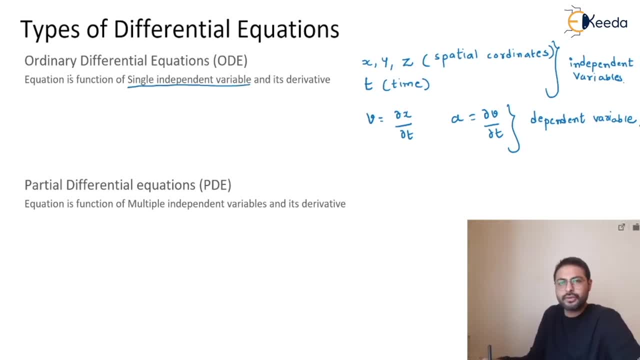 Then it is known as Ordinary differential equation. Let me give you one example. Here it is A spring mass system. Here the Mass M is attached With the spring, which is having K stiffness And it is oscillating in this direction. 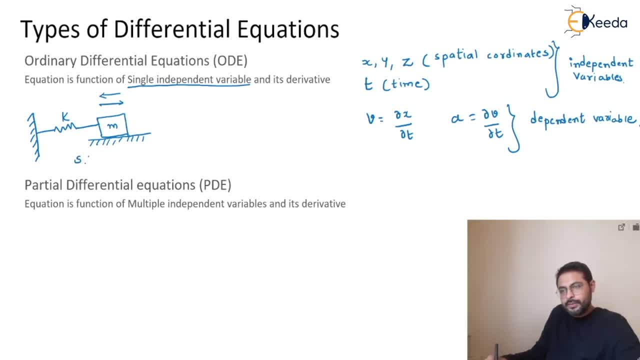 These two directions. So it is Nothing but the simple harmonic motion. And the motion Can be represented by Ordinary differential equation Like this. So here, As you can observe, in this equation, Here the direction is x If the spring is vertically. 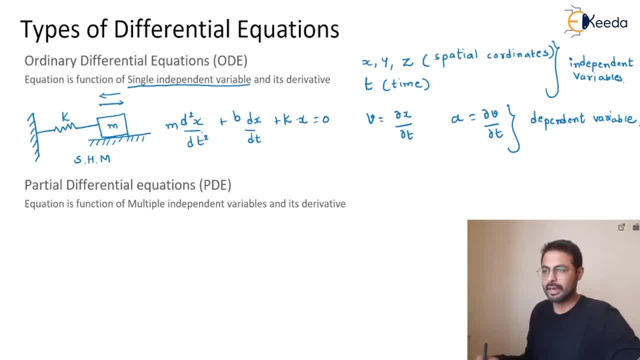 Hanged. Then instead of x We can write here y. So Here The Spring, Simple, harmonic motion Of a spring Depends On The time, T Only. So here Only one Single Independent variable. 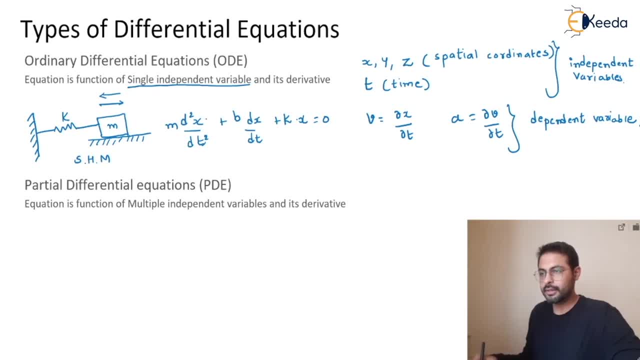 Is Present Inside The Equation, So it is known as Ordinary differential equation. So It is known as Ordinary differential equation. Now Let's understand What is Partial differential equation, So The Difference Between: 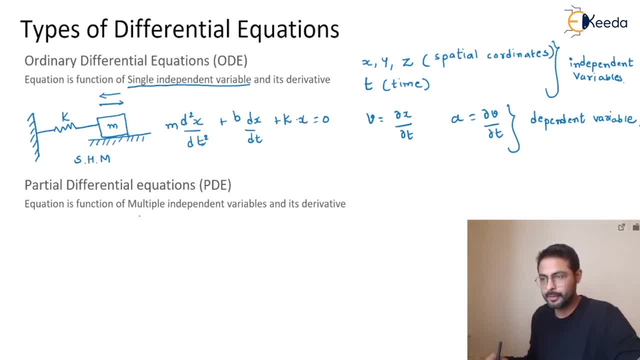 Ordinary differential equation And Partial differential equation Is Partial differential equation Is Having Multiple Independent Variable, So Instead Of Only One Independent Variable, This Is The Wave Equation, Or 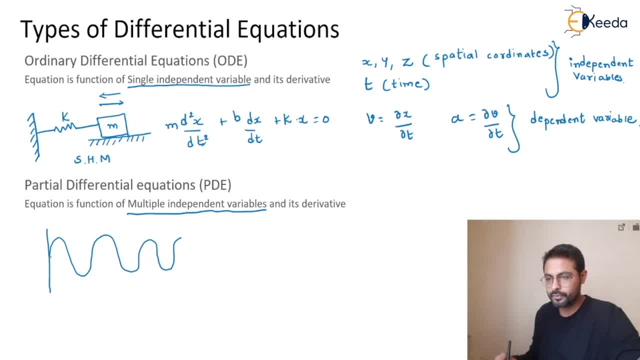 Wave Is Propagating, So This Axis Indicate The Time T And This Is The Amplitude Of The Wave In One Direction We Can Take. 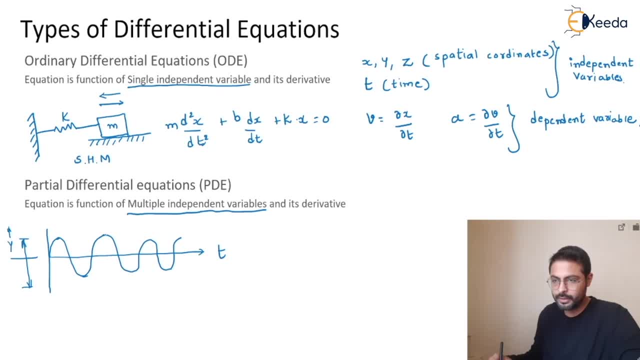 So Amplitude Is Changing Over Time Like This. So If We Want To Represent The Wave Equation Of This Wave Supposed By You, So You 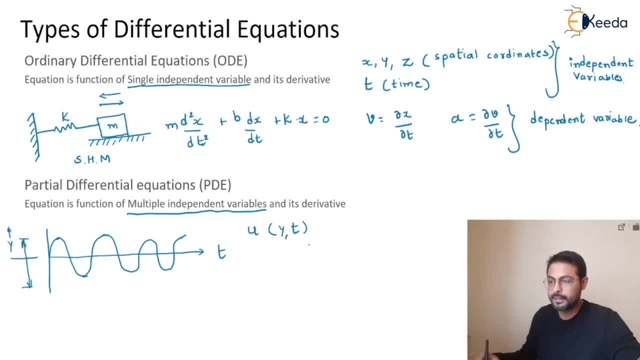 Will Be The Function. It Can Be Represented Like Del U By Del T, Equal To Alpha Del U Square By T Square. So Here: 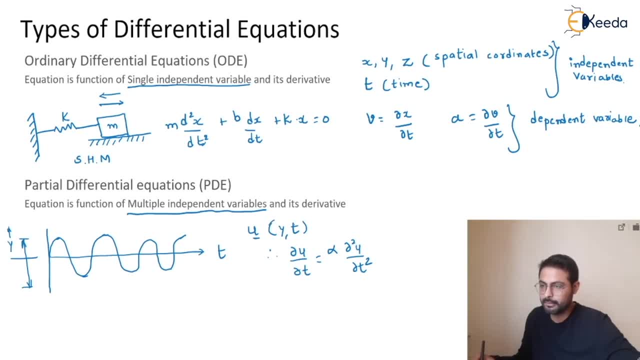 You Can See The Equation Or The Function As Partial Differential Equation. So Here The Difference Between Ordinary Differential Equation And Partial Is It Is Having. 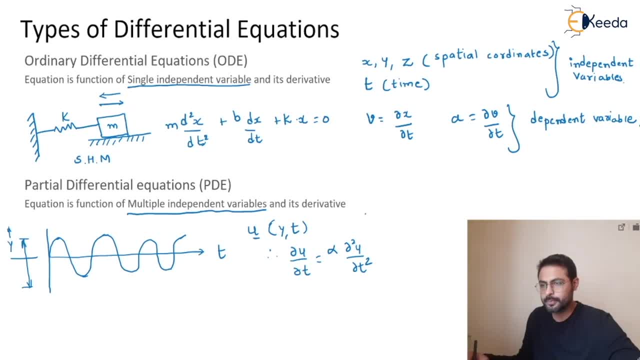 Multiple Independent Variable, While Ordinary Represents Only Single Independent Variable. So This: We Are More Concerned About Partial Differential Equation And Let's Understand Partial Differential. 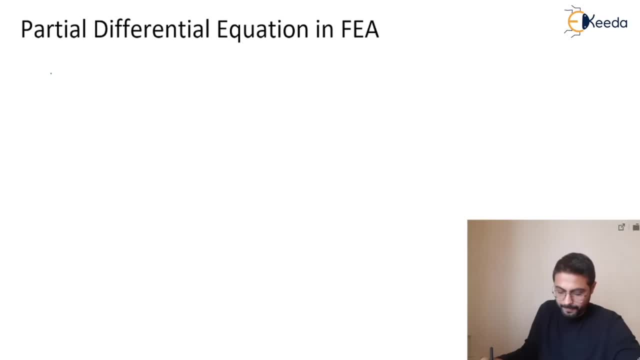 Equation In Depth By One More Example. So Suppose We Are Heating One Which Is Having A Regular Cross Section Area. Circular Regular Cross Section Area. 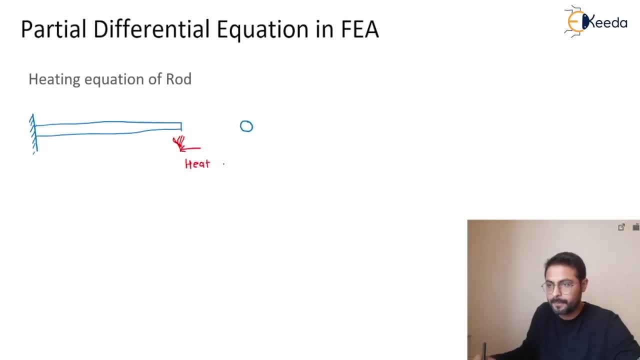 And We Are Heating From Here. So This Is The Heat Source And This Rod Is Having Nothing But The Temperature Capital T, So Temperature Will. 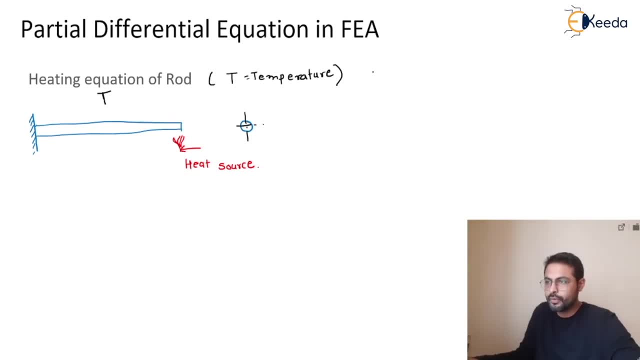 Get Changed Over Time. So Small T Is Nothing, But The Time And If We Consider This Direction. So Now We Want To Represent How The 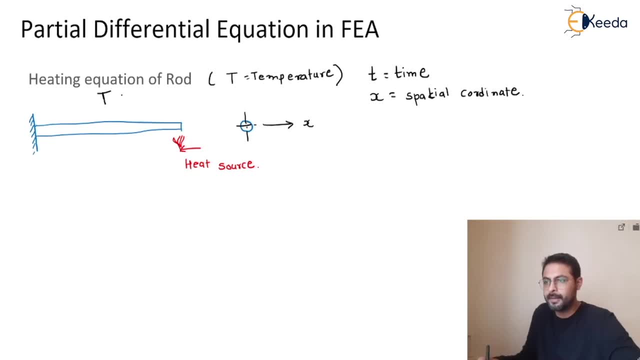 Temperature Is Changing Over Time, And As Well As It Will Change Over Various Points Like This. So Here We Are, Taking As Well As At: 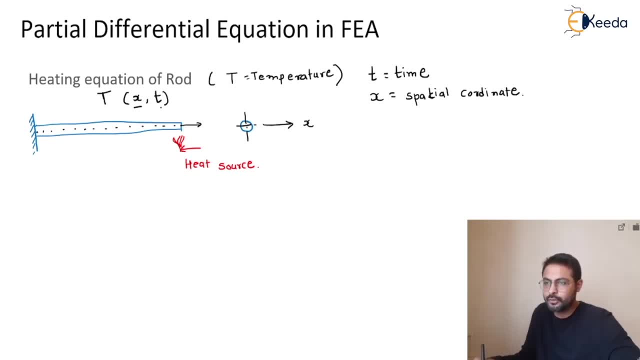 Different Time, The Temperature Will Be Different. So This Temperature Is A Function Of Two Independent Variable. First Is A Spatial Coordinate And Second Is The 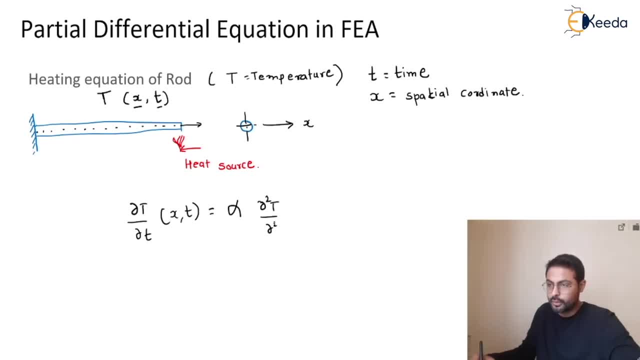 Temperature, Which Is The Material Property Of Body. The Rod Is Made Up Of Some Material And Alpha Is The Material Property Which Indicates The Conductivity. 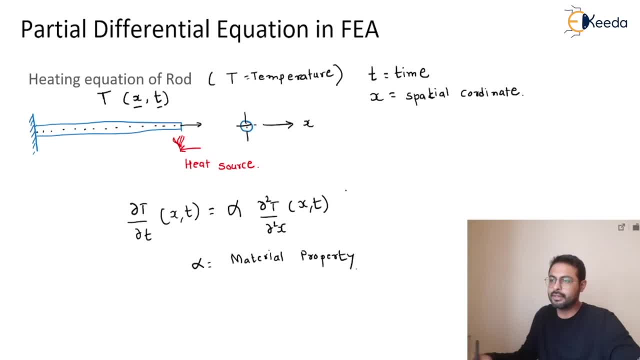 Of The Material Is Having More Than Two Independent Variables, That Is, X And T. So It Is Denoted By Partial Differential Equation And It 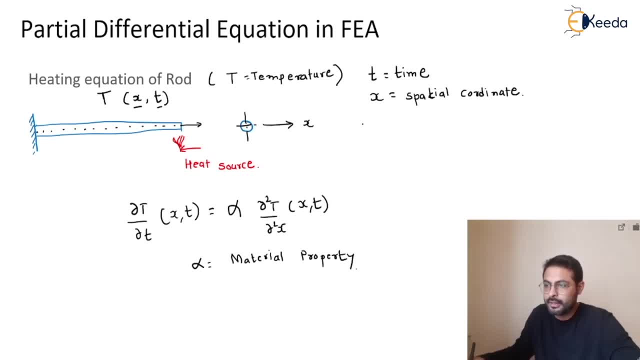 Is Having Derivative Of It. So This Is A Form. If This Rod Is Having A Per Cross Section Area, Then We Have To Consider: 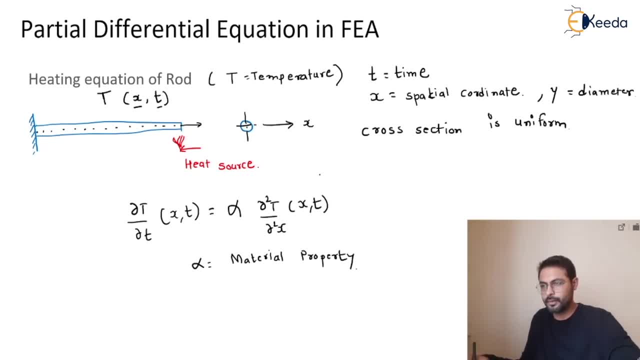 One More Special Coordinate, That Is Y, Which Is Related To Regular Cross Section Area. So To Understand It More, Let Me Give You One More. 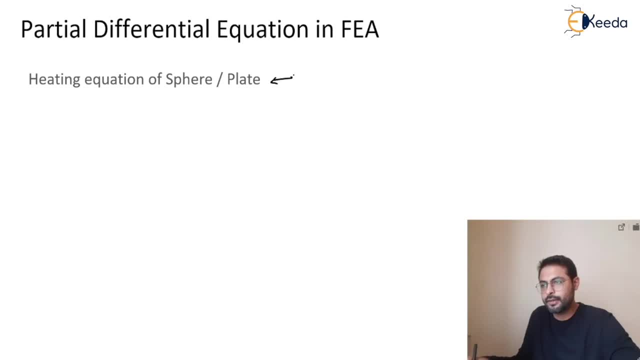 Example Of Partial Differential Equation, Like Heating Of The Sphere Or Plate. So Here You Are, Compiling The Three Dimensions, So It's A Three D. 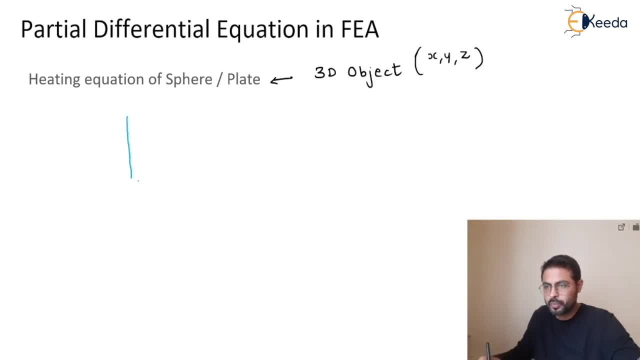 Object, And Now We Are Going To Consider This Three D Object. So We Are Submerging A Metal Body Which Is A Shape Of This. 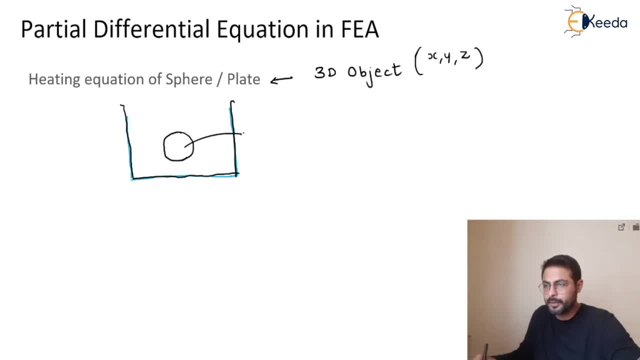 Is The Sphere Sphere And It Is Submerged Into A Hot Water, And It Is Submerged Into A Hot Water And It Is Submerged. 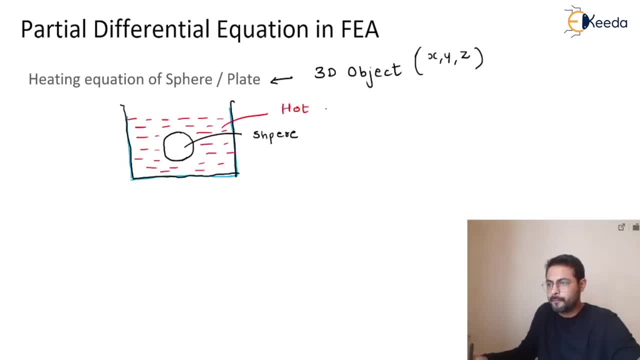 Into This Sphere. So How This Sphere Is Getting The Heat From Hot Body To Cold Body That We Have To Represent. So We Have, We. 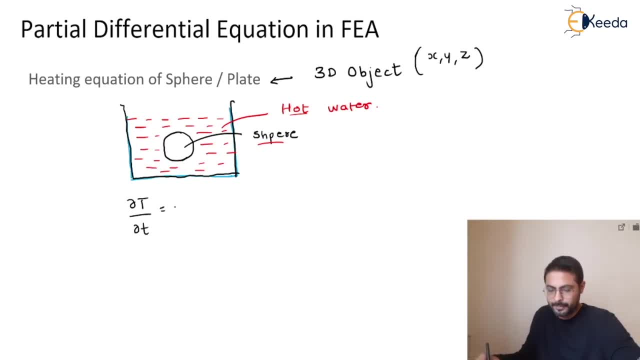 Can Represent It Like This: Is A Function Of Conductivity And Three Dimensions Of A Body: Del Square T By Del Y Square Del Square.